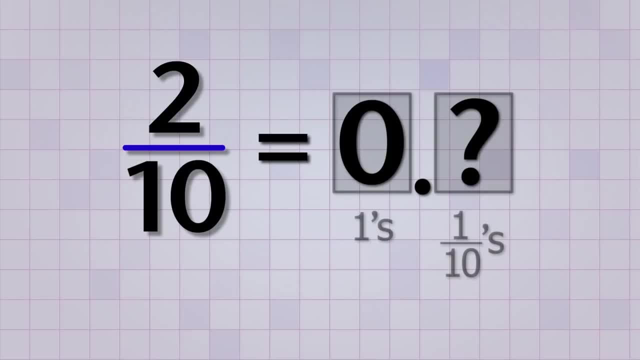 have 2 over 10 instead. Well, all we have to do is change the digit in the tenths place to a 2.. So 2 over 10 equals 0.1.. In fact, we can keep counting tenths like this: 3 tenths, 4,, 5,, 6,, 7,, 8,, 9, and finally. 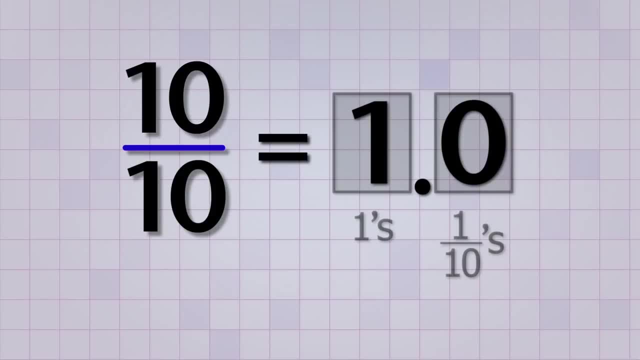 10 tenths. But look what happened when we got to 10 tenths. Now we don't have a digit for 10, so we had to use the next number place over the ones place. But that makes sense because if you have the fraction 10 over 10, that makes a whole and the value is just 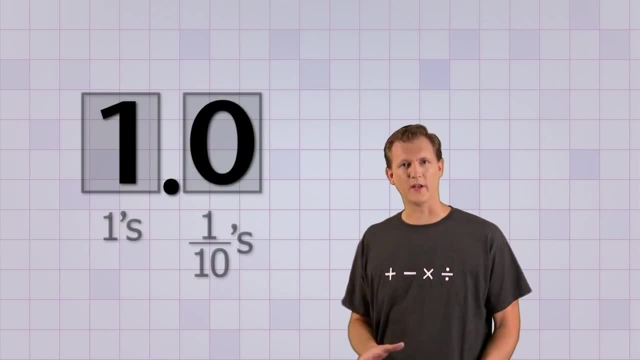 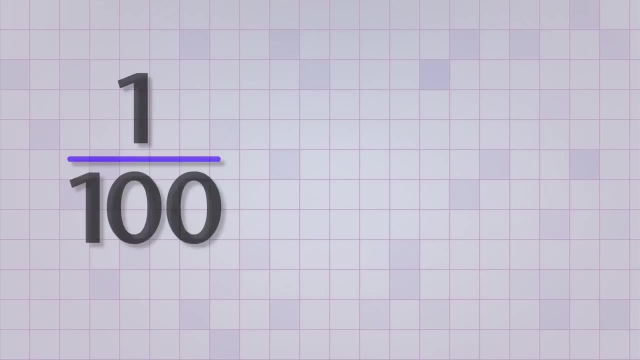 1.. Of course we don't really need the 0 in the tenths place to write 1,, but as long as the decimal point's there, at least we won't confuse it with 10.. Tenths are pretty easy, but what about hundredths? Let's start with the hundredths building block. 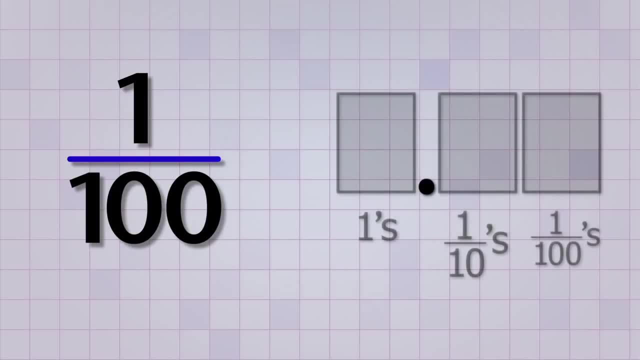 1 over 100.. To write that as a decimal, we simply put a 1 in the hundredths place. We also need to put a 0 in the tenths place to act as a placeholder and show that we have no tenths. And we still need to put a 0 in the ones place, as usual. 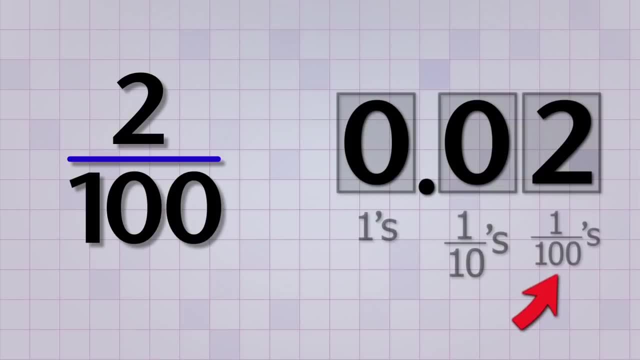 Next, let's try two hundredths. For that, we simply put a 2 in the hundredths place. Let's keep on counting with hundredths, just like we did for tenths, 3 hundredths, 4,, 5,, 6,, 7,, 8,, 9, and 10.. 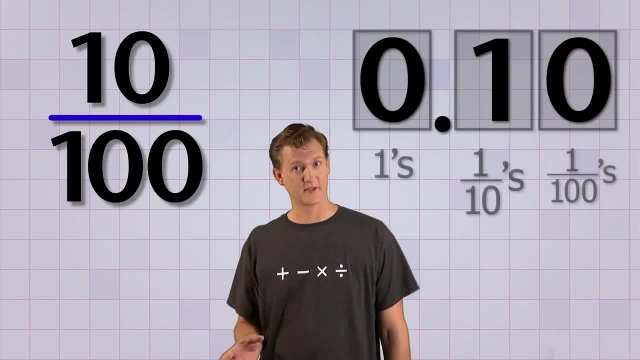 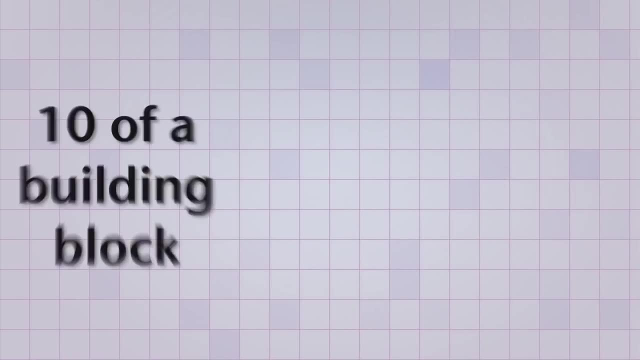 Ten hundredths, Ah, but look what happened when we got to ten hundredths. Just like before, we have to use the next number placed to the left, the tenths place. This happens because any time you have 10 of a building block, they combine to form. 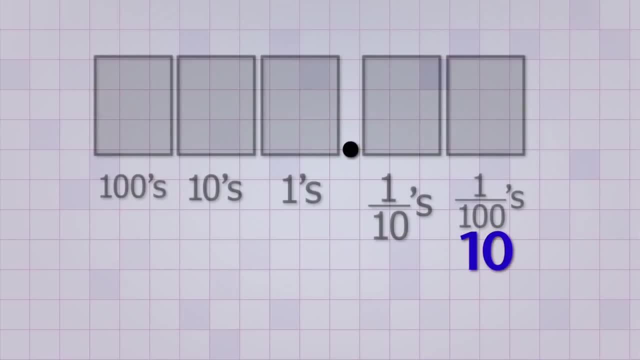 1 of the next biggest building block. For example, ten hundredths is a tenth, ten tenths is a 1,, ten ones is a 10, and ten tens is a hundred. Now, the next fraction after 10 over 100 is 11 over 100.. Now, if you think about it, you'll 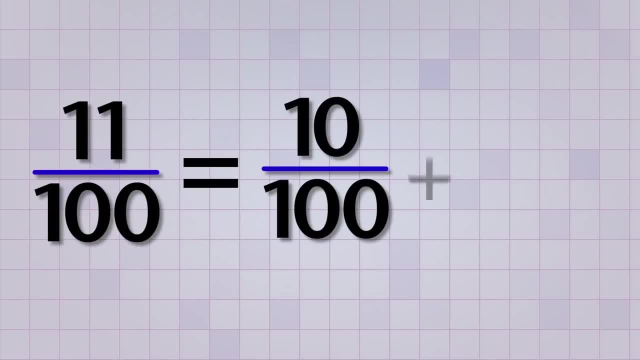 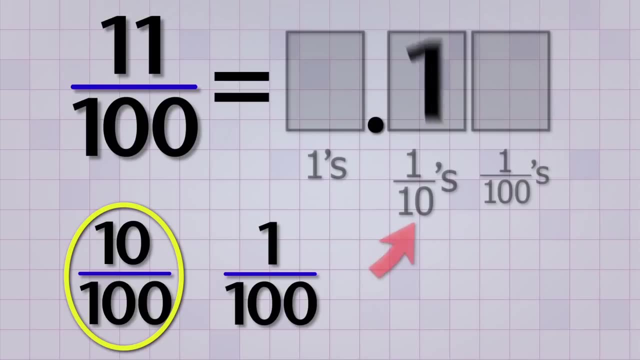 see that 11 hundredths is really just a combination of ten hundredths and one hundredth. Knowing that will help us write it as a decimal, Because a group of ten hundredths is equal to one tenth. we put a 1 in the tenths place And we still have that one hundredth left over. 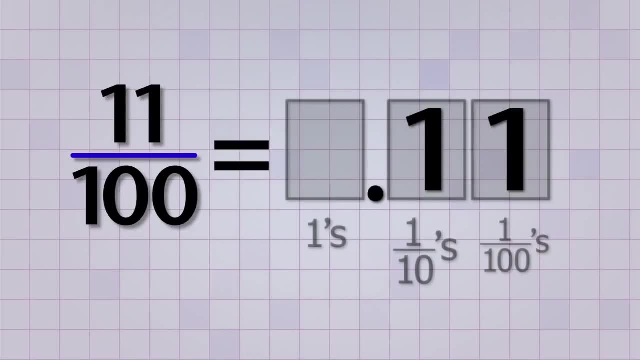 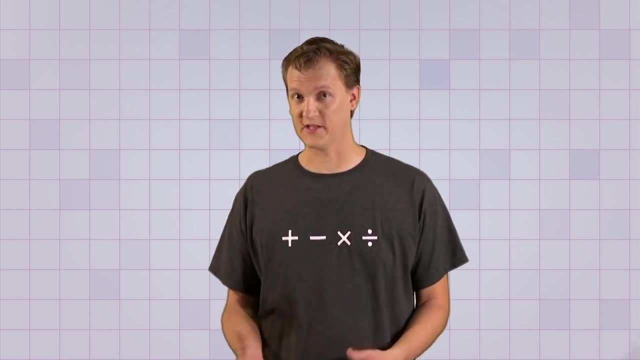 so we put a 1 in the hundredths place There, 11 over 100 is just 0.11 as a decimal. Fortunately, you don't have to break up the fraction into tenths and hundredths each time. Any time you have a two digit number over a hundred, all you have to do is put those. 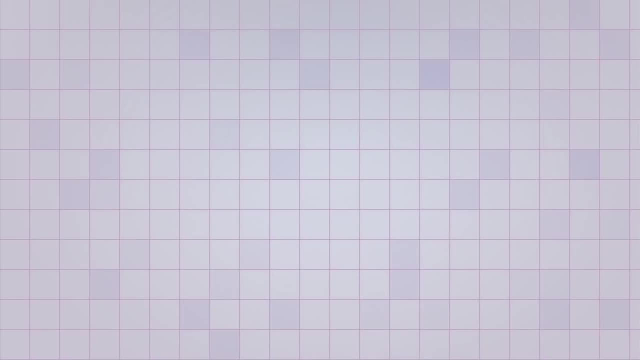 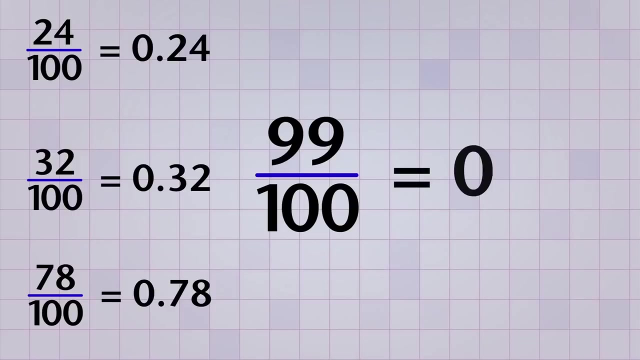 into the tenths and hundredths place of your decimal number. Let's look at a few more examples to help you see the pattern. 24 over 100 would be 0.24.. 32 over 100 would be 0.32.. 78 over 100 would be 0.78.. And 99 over 100 would be 0.99.. 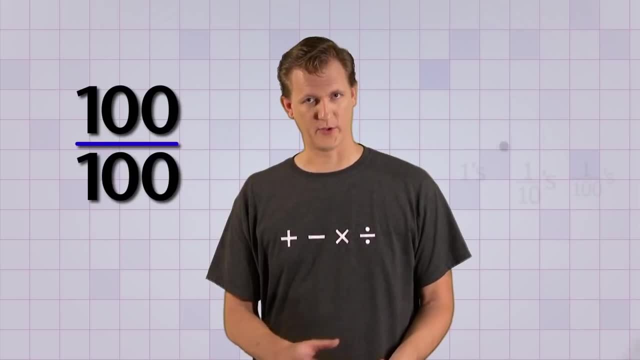 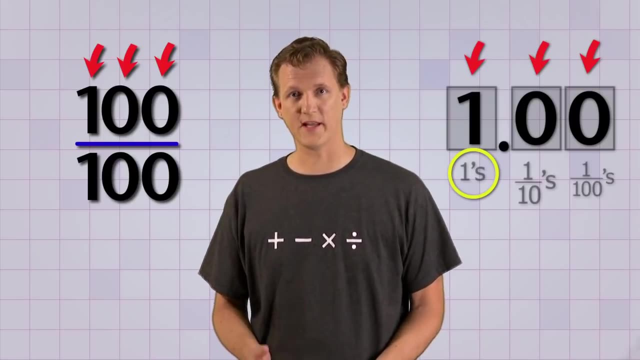 Now what do you think will happen if we convert the fraction 100 over 100 into a decimal Right? A hundred has three digits, so we need to use another number place. Now, the next one over is the ones place, And that makes sense because 100 over 100 is a whole and its value is just 1.. 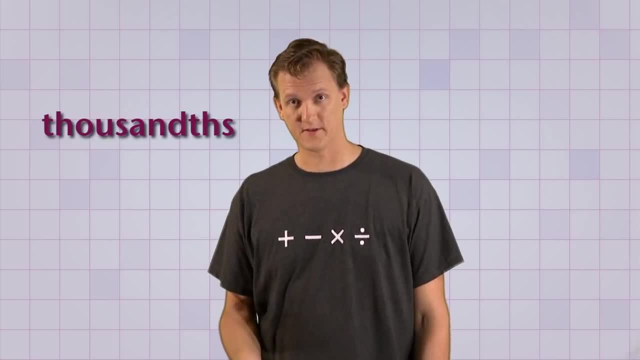 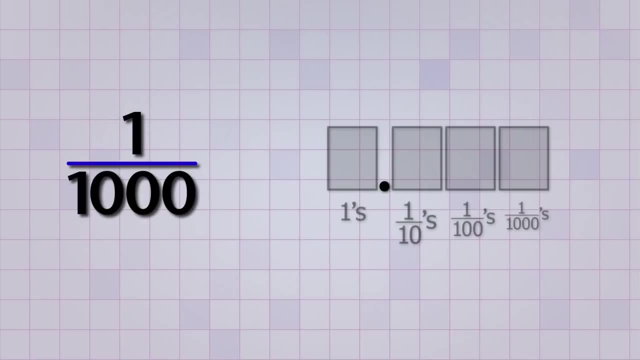 Now that we know how to convert hundredths into decimals, let's try converting thousandths, That's, fractions that have 1000 as the bottom number. Let's start with 1 over 1000.. Now, this should be easy. All we have to do is put a 1 in the 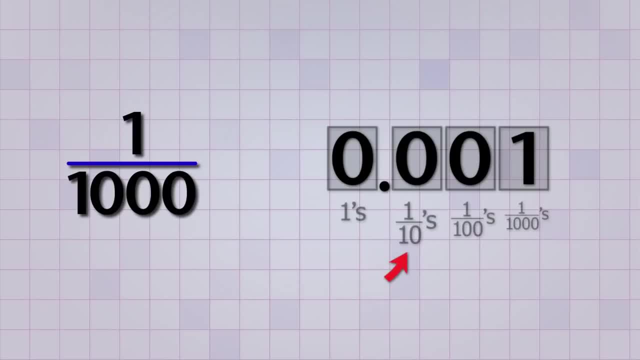 thousandths place. Notice that this time we need zeros in both the tenths and the hundredths place to act as placeholders. Next, let's try converting 10 over 1000.. Remember that 10 thousandths is the same as 100, so 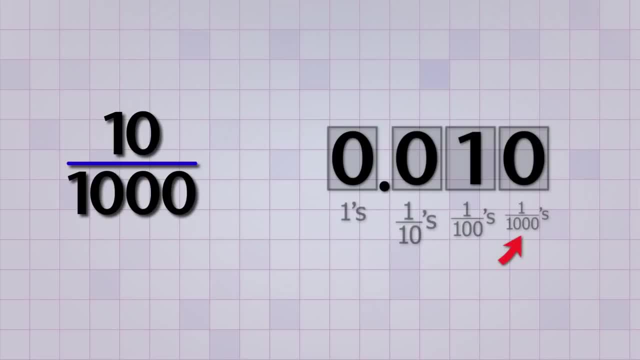 we'll put a 1 in the hundredths place and we'll put a zero in the thousandths place. We don't really need the zero at the end, but it helps us see that this was 10 thousandths. Alright, what if we have 100 over 1000?? Now, that's a three digit number on top, so we're. 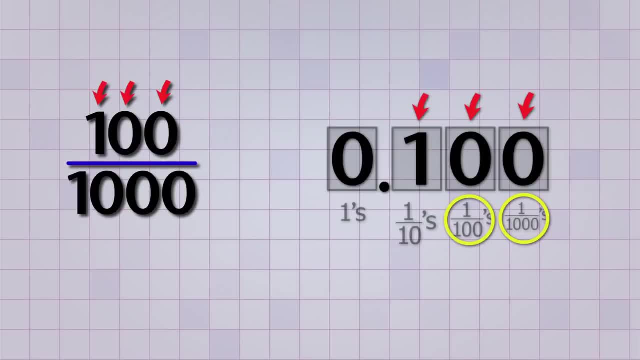 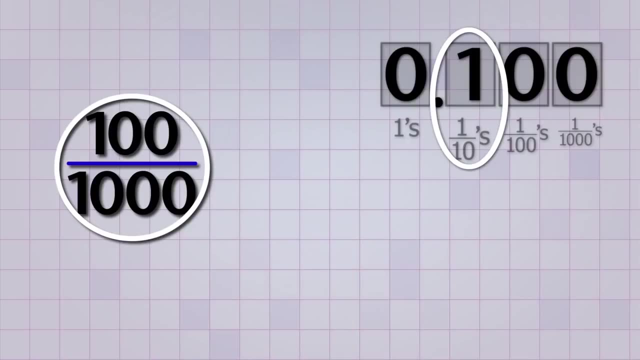 going to need to use three number places: The thousandths place, the hundredths place and the tenths place. So, as you can see, 100 over 1000 is just the same as 1 tenth. Let's see a few more examples. 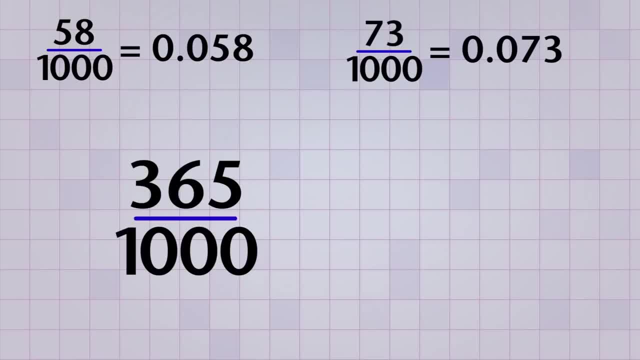 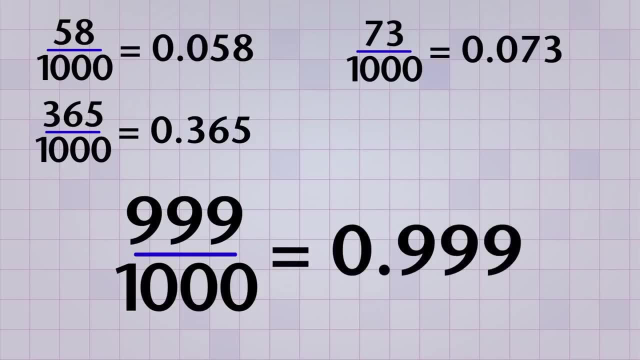 90 over 1000 is 0.073.. 365 over 1000 is 0.365.. And 999 over 1000 is 0.999.. And finally, what do you think we'd get if we converted a 1000 over 1000? Right again. 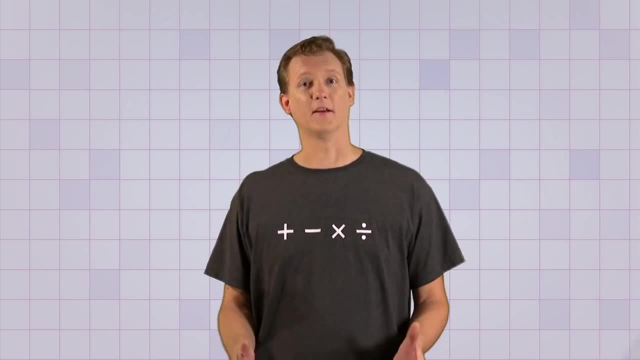 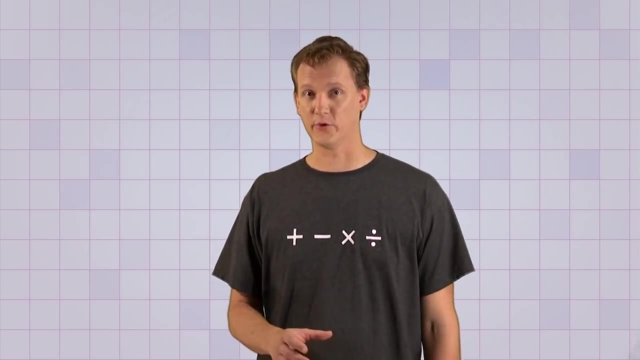 a 1000 over 1000 is just a whole, so it's value would be 1.. Ok, so we've learned how to convert base- trimming fractions into decimals, but we can go the other way too. We can start with a decimal and convert it into a fraction. 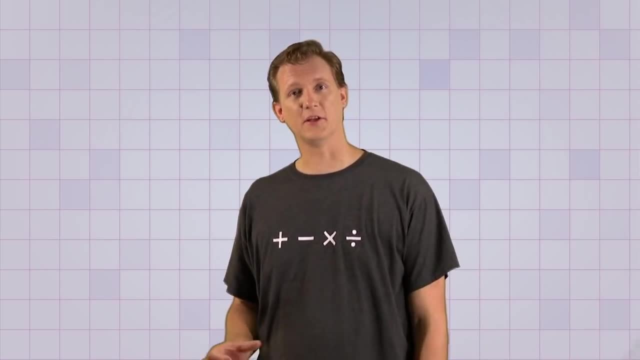 to convert a decimal number into a fraction, All we have to do is take the decimal digits and make them the top number of a base 10 fraction. The bottom number will be determined by the smallest number place used in our decimal. For example, to convert 0.8 into a fraction. 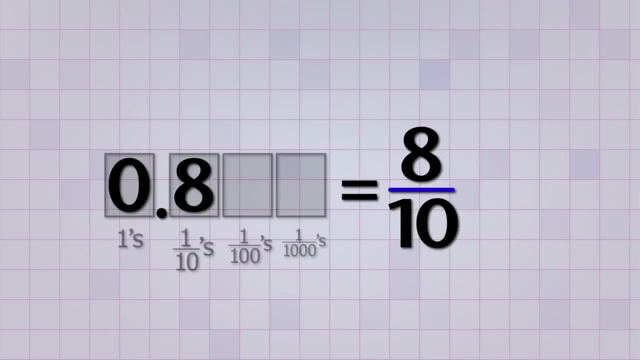 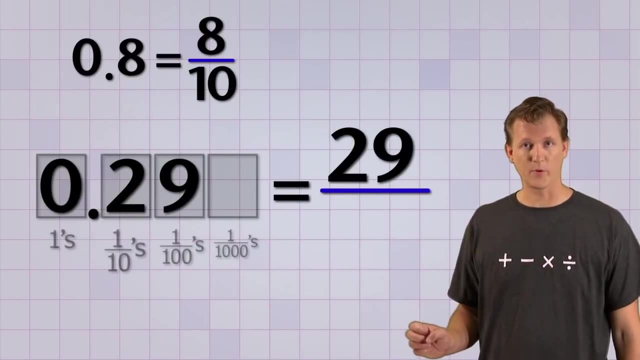 we put an 8 on the top and a 10 on the bottom because the smallest number place in our decimal was the tenths place. And to convert 0.29 into a fraction, we put a 29 on top and we put a 100 on the bottom, because the smallest number place in our decimal was the hundredths. 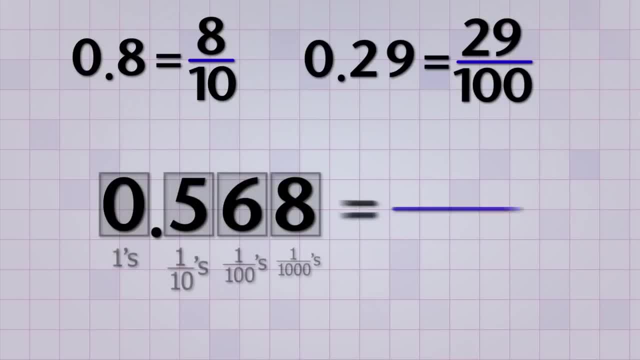 place. And finally, to convert 0.568 into a fraction, we put 568 on top and a 1000 on the bottom, because the smallest number place in our decimal was the thousandths place. Okay, so far all of the fractions that we've converted to decimal numbers, and vice versa. 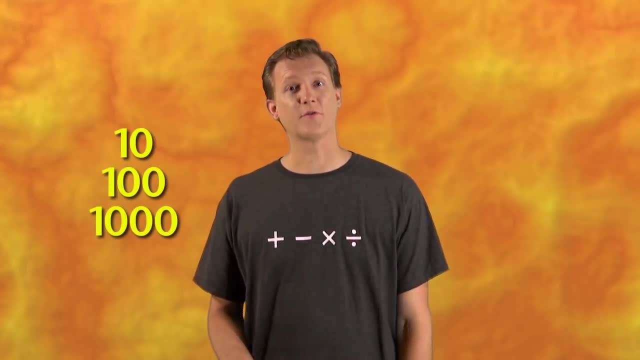 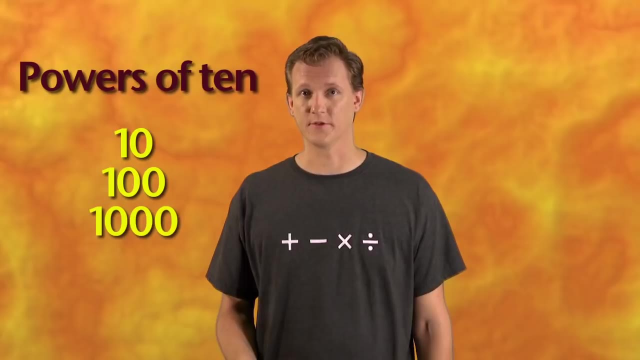 have bottom numbers like 10,, 100, or 1000.. Those fractions are easy to convert because our number system is based on powers of 10.. We have number places that we can convert to decimal numbers and vice versa. We have number places specifically for counting those. But what if we want to take fractions with? 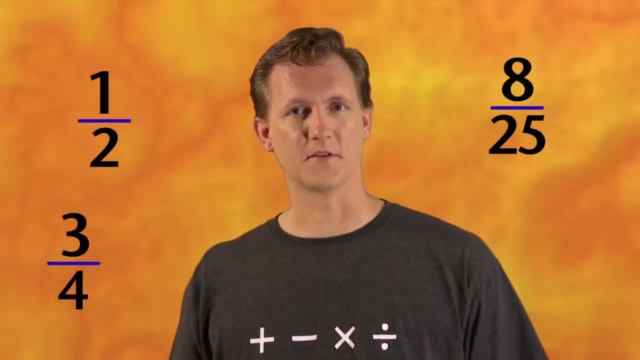 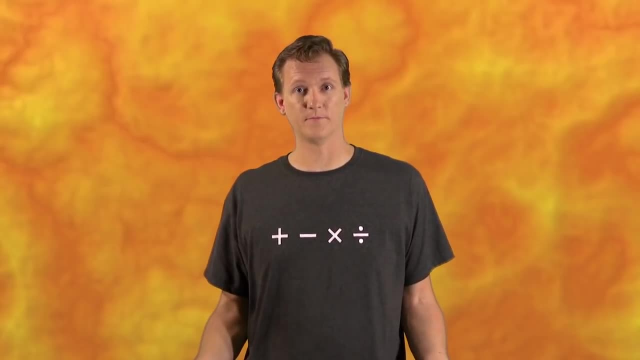 different bottom numbers like 1, half, 3, fourths or 8, twenty-fifths, and write those as decimal numbers. We don't have special number places for halves, fourths or twenty-fifths. So what are we going to do? Well, you're going to have to watch the next section to find. 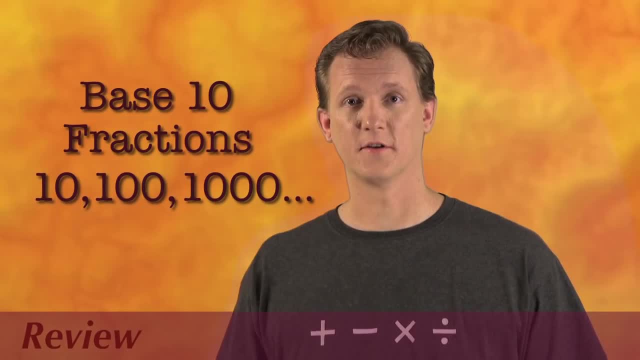 out. But first let's take a minute and review all this. If a fraction has a bottom number that is, a power of 10, then it's easy to convert it into a decimal number because there are number places just for counting base 10 fractions. 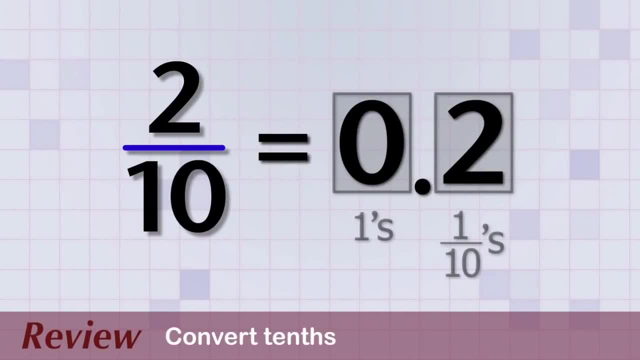 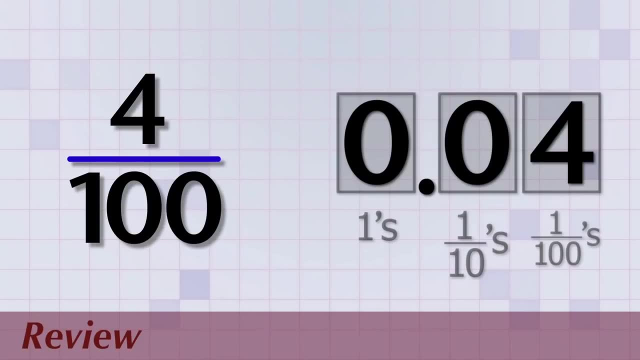 To convert tenths, all you have to do is put the top number in the tenths place. To convert hundredths, you have to use both the tenths and the hundredths place together. To convert thousandths, you have to use three number places, and so on. You can also convert. 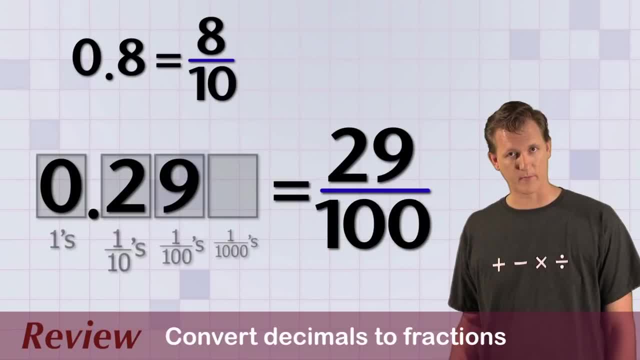 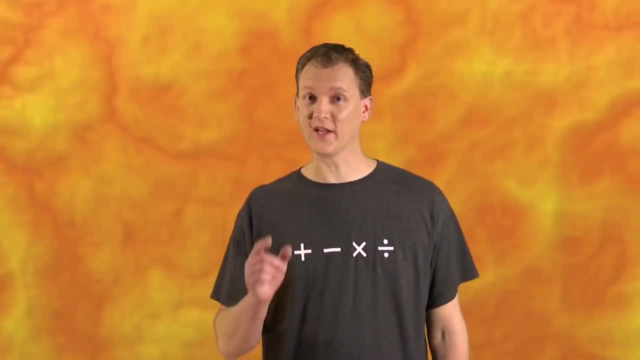 from a decimal number to a fraction just by making the decimal digits the top number of the fraction and by using a bottom number that's based on the smallest number place from our decimal. Be sure to do the exercises so you get really good at converting base. 10 fractions.